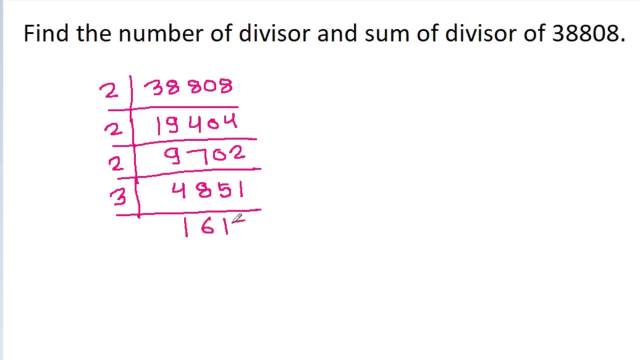 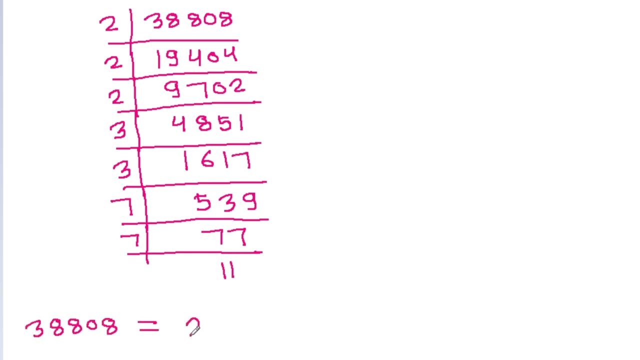 And 3 times 1,, 6,, 1, 7.. And 3 times 5,, 3 and 9.. And 7 times 7,, 7 and 7 times 11.. So 38808, it is 2 Q times 3, a square times 7, a square times 11.. 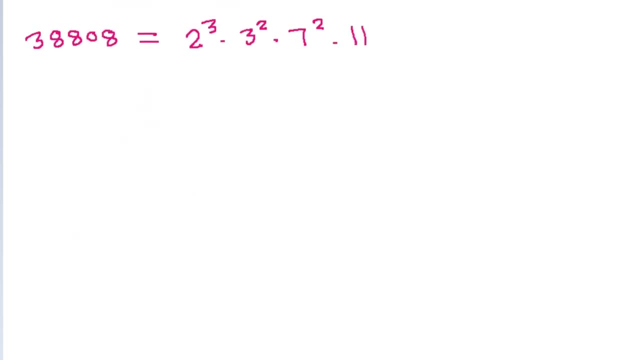 And 7 times 11.. And 7 times 7, 7,, 7 and 7 times 11.. number of divisor: it will be equal to this: 3 minus 1 times 2 minus 1 times 2 minus 1, and this 1 minus 1, and it is 4 into 3 into 3 into 2 and 4 into 3, is 12. 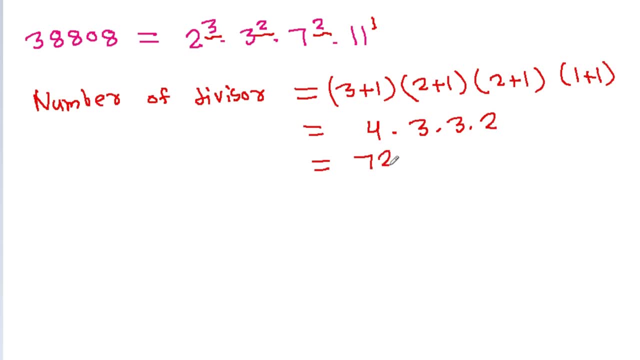 times 3 is 36, times 2 is 72 and 38808 is 2 cube, 3 square, 7 square and 11 power 1. so sum of divisor it will be equal to. we have 2 cube, so it will be 2 power 0. 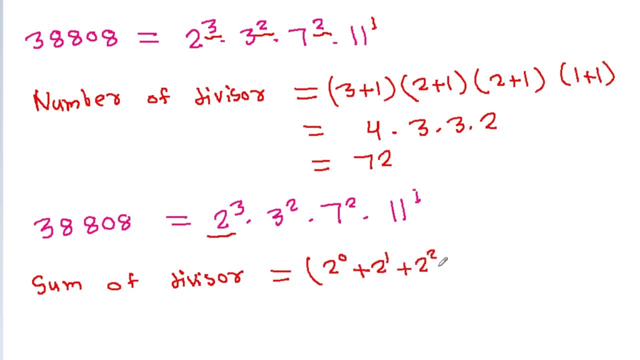 and minus 2 power 1 minus 2 power 2 minus 2 power 3 times. we have 3 square, so it will be 3 power 0 minus 3 power 1 minus 3 power 2 times and we have 7 power 2, so it will be 7 power 0. 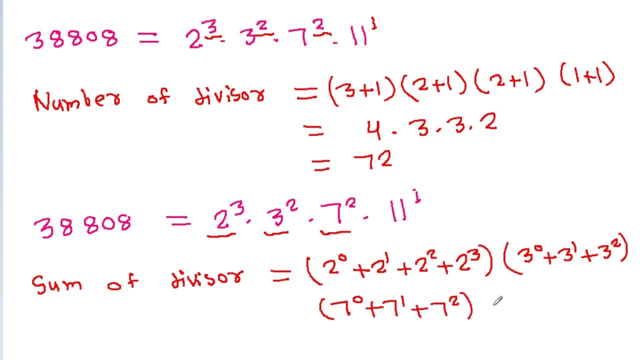 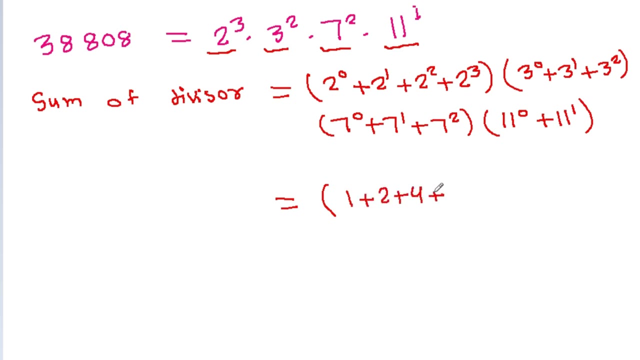 minus 7 power 1 minus 7 power 2 times, we have 11 power 1, so it will be 11 power 0 minus 11 power 1, And it is 1 plus 2 plus 4 plus 8 times 1 plus 3 plus 9 times 1 plus 7 plus 49 times 1 plus 11..